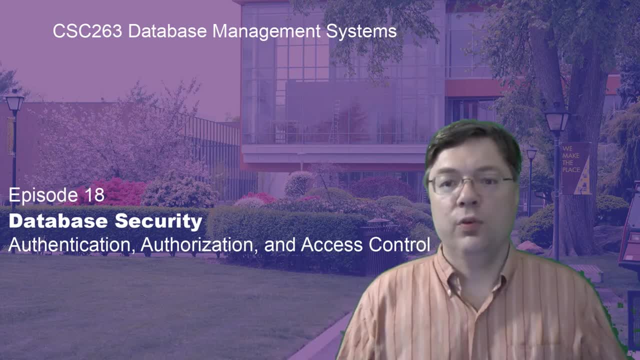 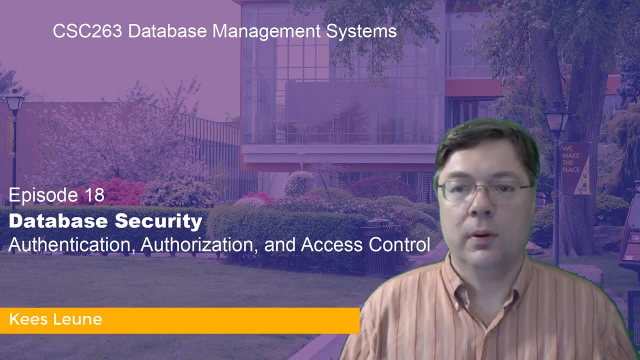 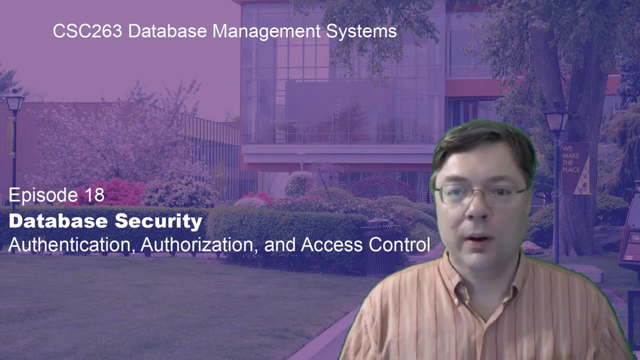 Hello, welcome to another episode in CSC 263, Database Management Systems at Adelphi University. Today we'll continue our conversation about database security. In the previous video I briefly introduced what security is all about. It's all about maintaining the confidentiality. 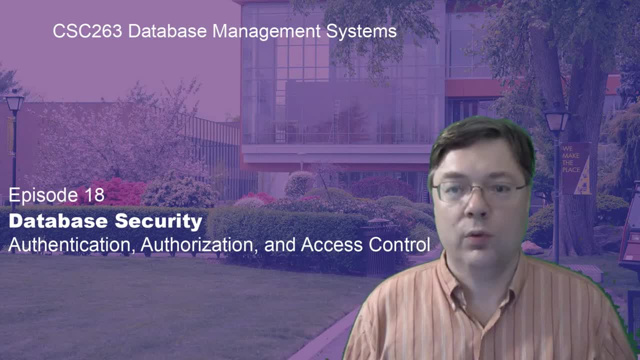 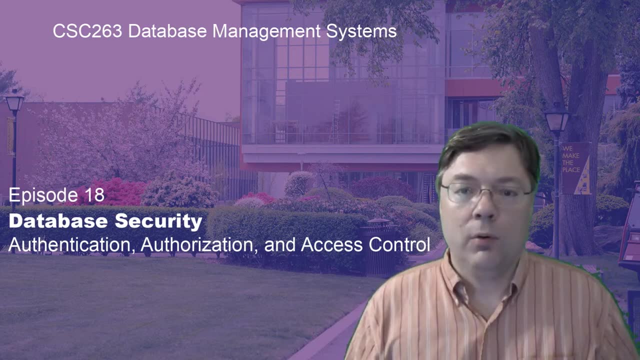 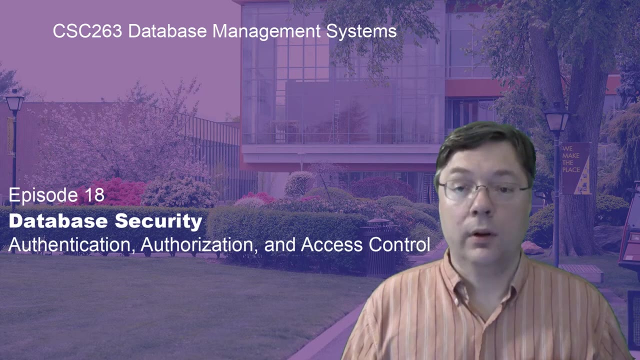 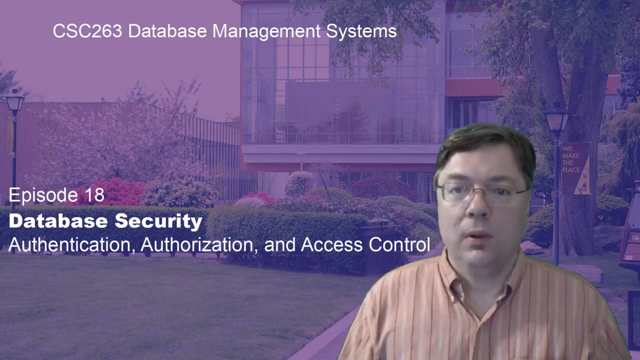 the integrity and the availability of the data stored in our databases. We saw that the database management system has three main control types that it can deploy: Authentication, access control, cryptography and audit. Today, we'll talk a little bit more detail about what authentication means. 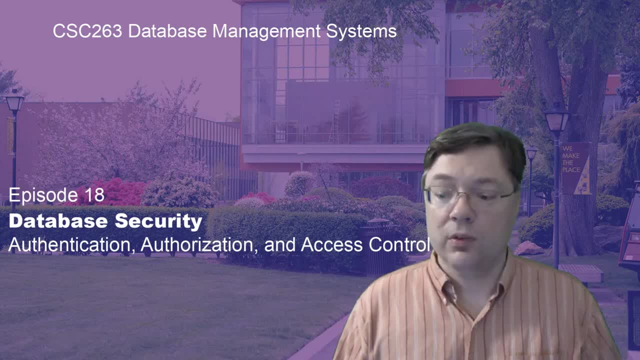 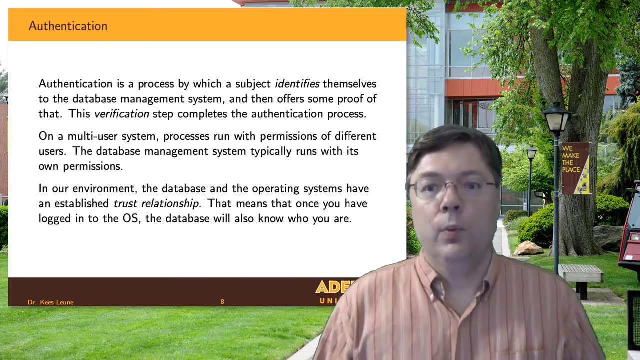 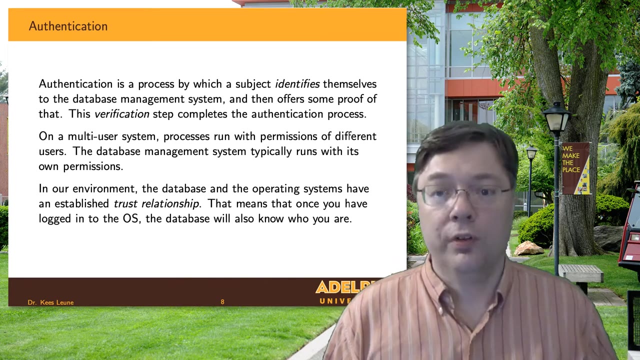 for a database management system and for computer systems in general. So when we look at cybersecurity as a discipline, we often begin by explaining that identification plus verification makes authentication And it basically means common sense If we have to interact with someone and they claim an identity. 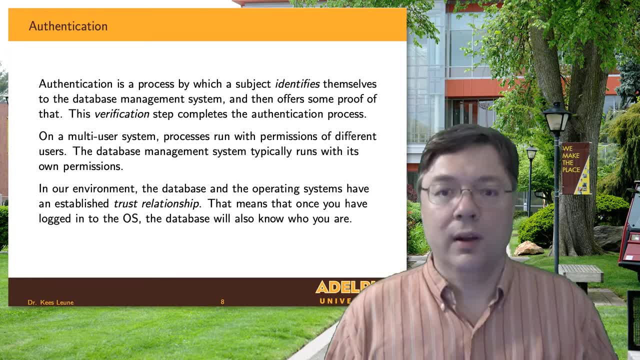 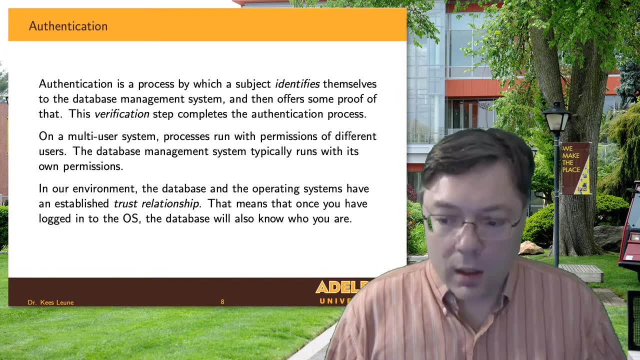 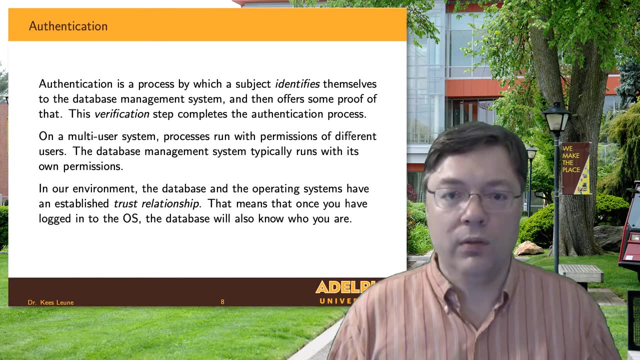 we're going to ask them to provide some form of evidence of that identity. How do we know that this person is actually who they claim to be? The same thing has to happen for a database, Since a database regulates access to individuals based on who they are. 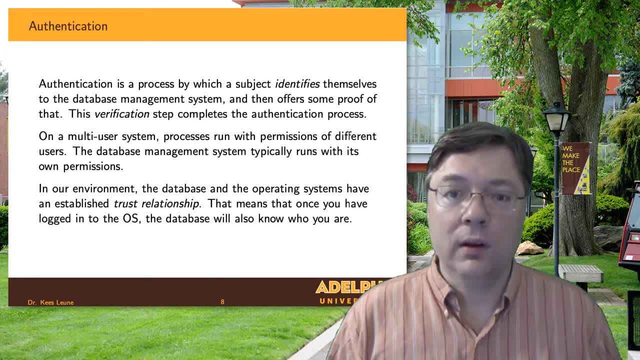 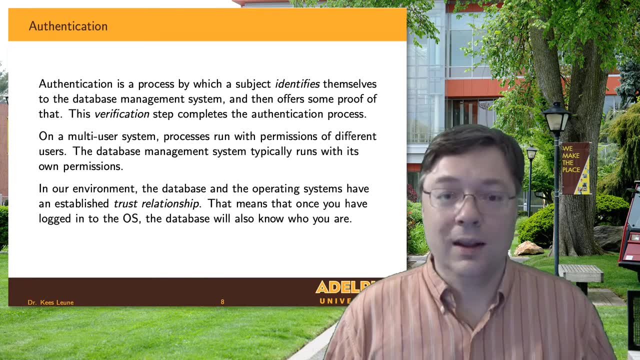 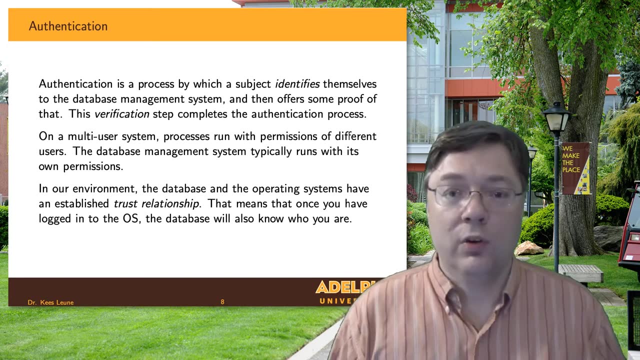 the database has to have a way to figure out who is using the database. This is prompted by the fact that a database management system provides concurrency, network-based access for multiple users at the same time, And in order to manage all of that and to maintain security, 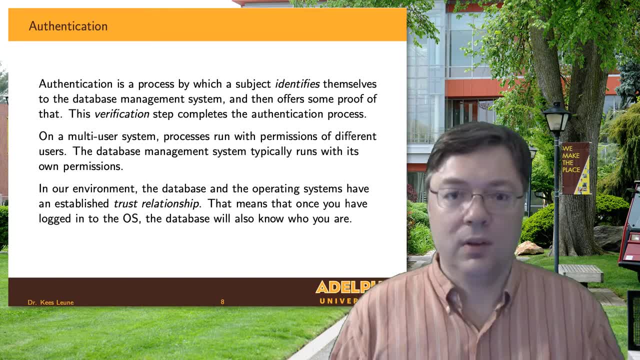 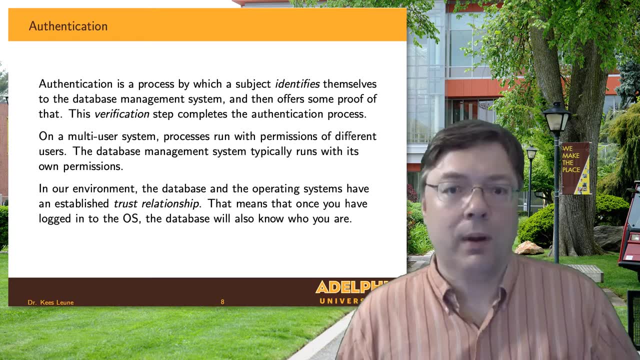 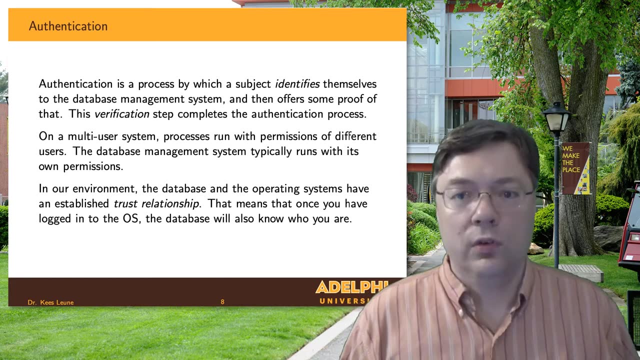 we have to know who each individual that interacts with the database is. Now, there's different ways we can do this. Traditionally, username and password for a network-based service is an easy way to do things, But that also brings with us a lot of other concerns with regards to security. 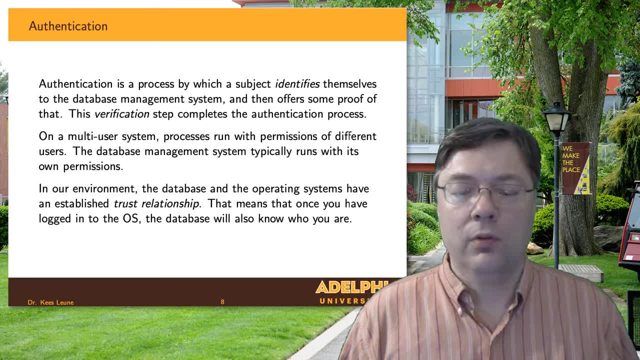 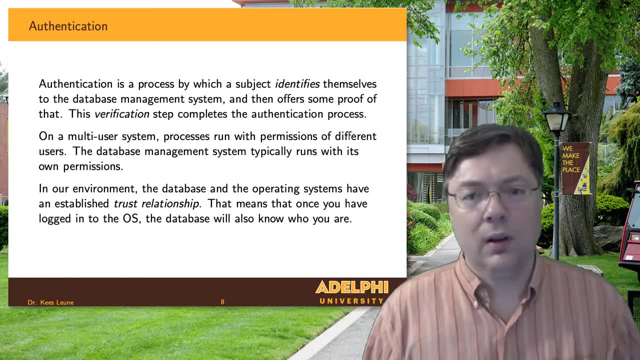 At this point we'll have to worry about network security, about transport level encryption, about making sure that there is firewalls in place and all kinds of stuff that we might touch on a little bit later on, but we're not going to go into a whole lot of detail about that. 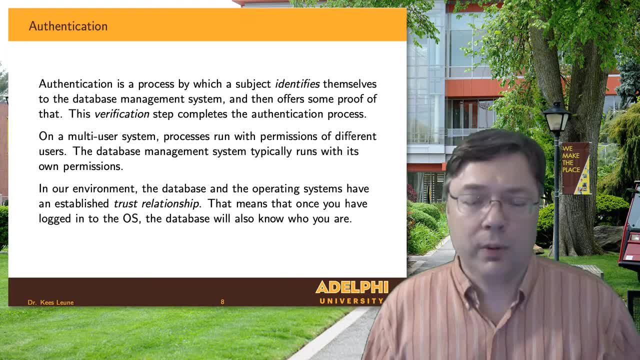 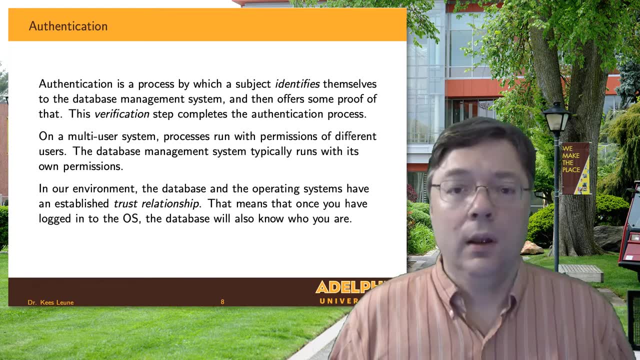 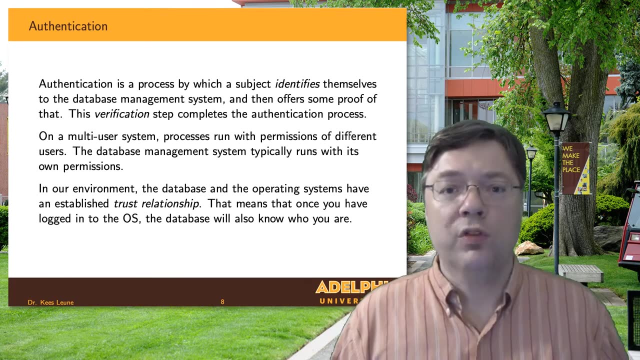 For our situation. for the practicum component of this course, we use the PostgreSQL database And we are actually connecting directly to the server on which the PostgreSQL database is running. So there's no separation in terms of different operating systems, different network hosts. 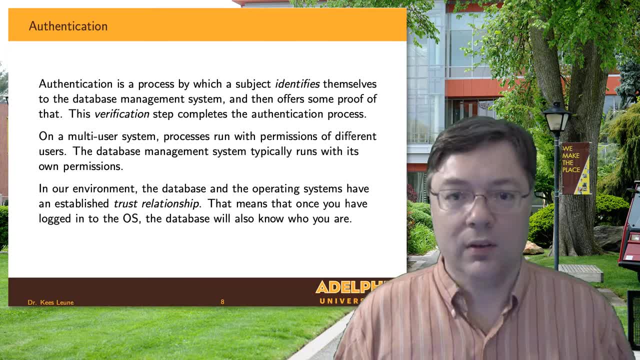 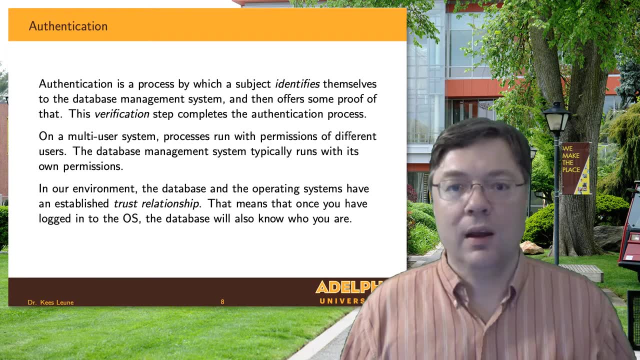 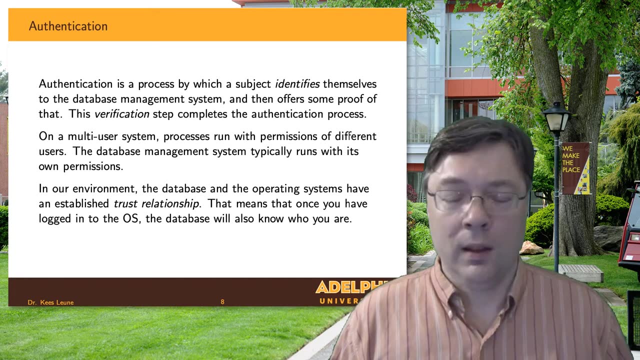 Everything is self-contained within the same operating system, And that gives us the benefit that we can almost delegate the authentication activity down to the OS. The OS already knows who you are, You know. if the OS doesn't know who you are, we're kind of stuck in the first place. 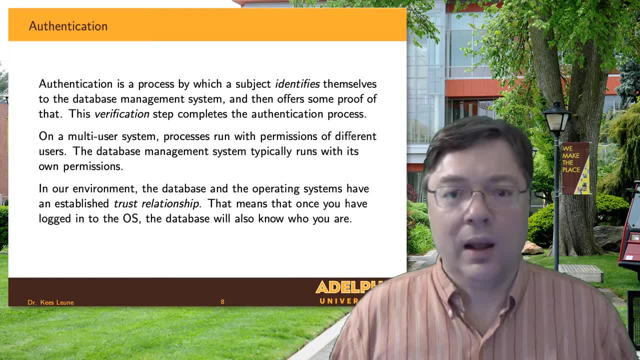 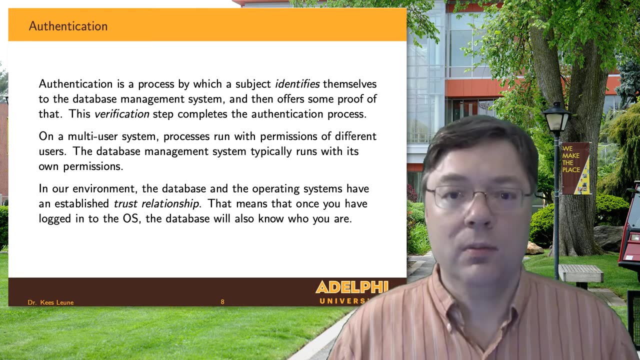 So the way that PostgreSQL is configured in our lab environment is that it will trust the operating system. So if I log in with my username and password to the operating system, the OS knows who I am At that point. the database management system is also going to be used. 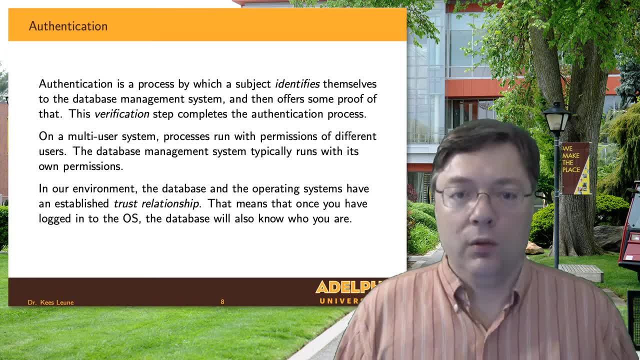 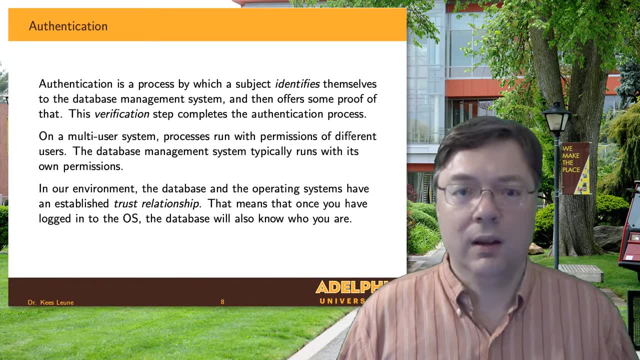 To be aware of who I am. It means that if you log into the database, you have a different way to log in, whether it's username and password or some form of a private key authentication. Either way, the OS knows who you are. 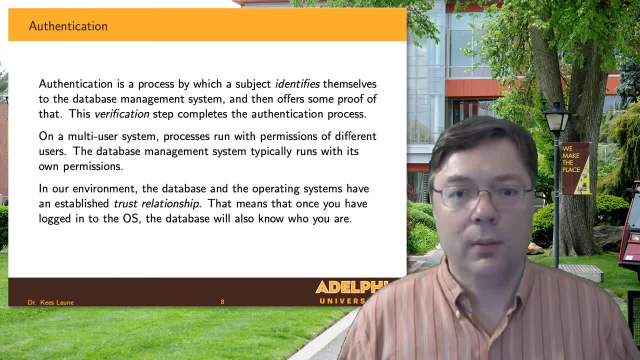 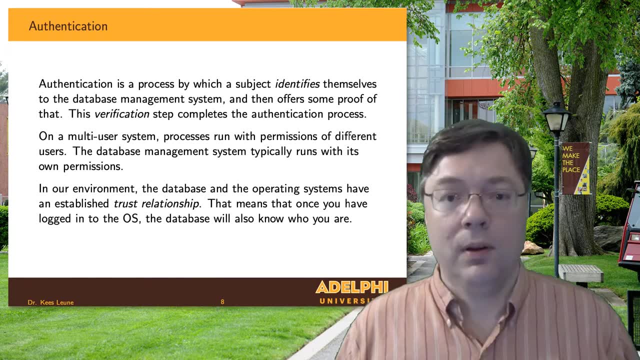 Otherwise you wouldn't be let in. When you connect to the database, you're connecting with your privileges and your credentials, And that means that by default you have no access to my databases unless I give that access to you, And that is, of course, called access control. 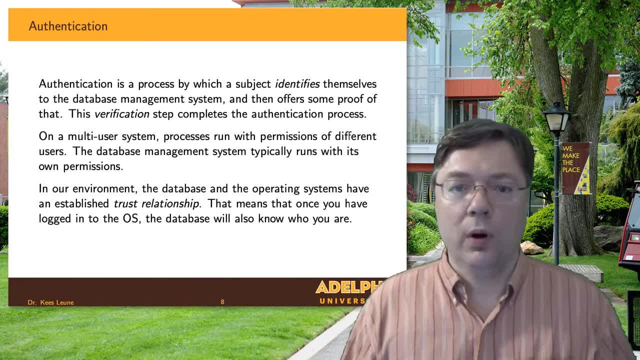 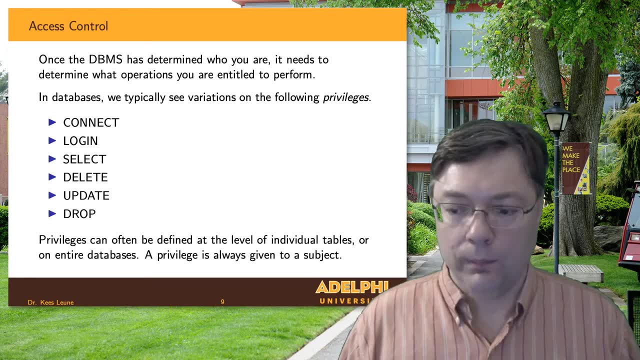 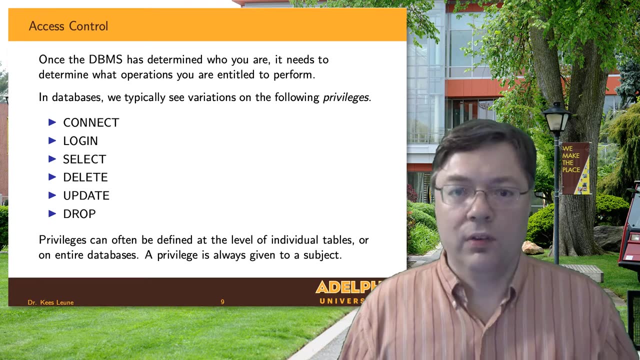 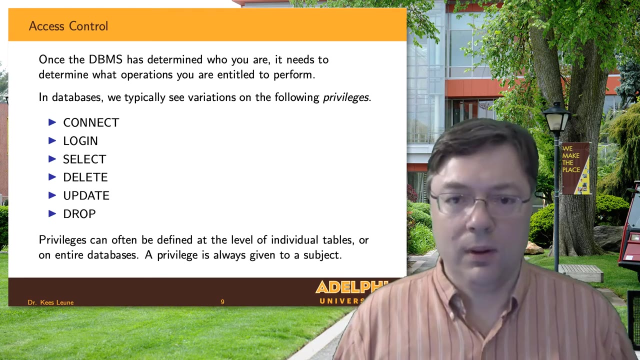 But identifying who you are and then using that to make decisions. that's the job for authentication and access control. There's actually a number of times throughout the DBMS operations that it needs to be able to know who you are and what rights you have to interact with the database. 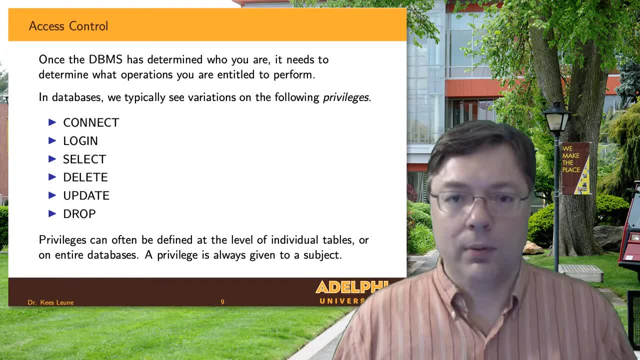 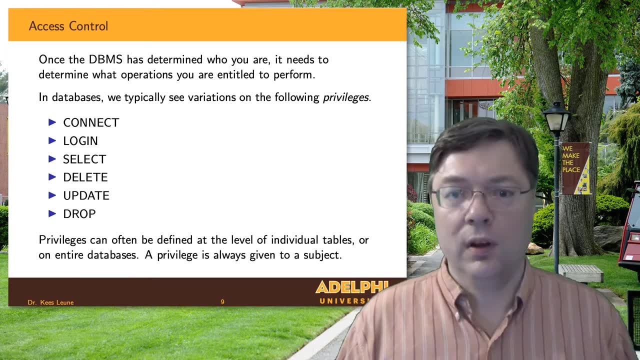 Because knowing who you are is just the first step. The next one is giving you specific information. The next one is giving you specific information. The next one is giving you specific information. The next one is giving you specific authorizations to say: okay, you are allowed to connect to the database using an interactive session. 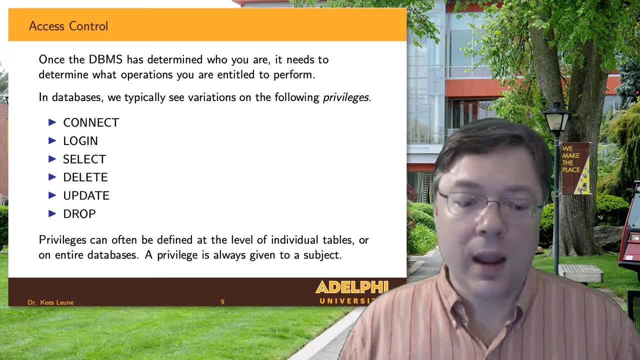 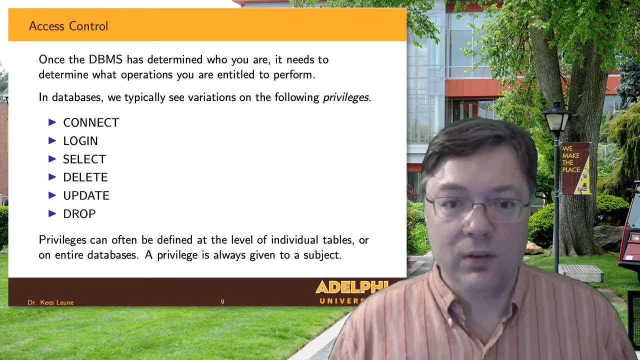 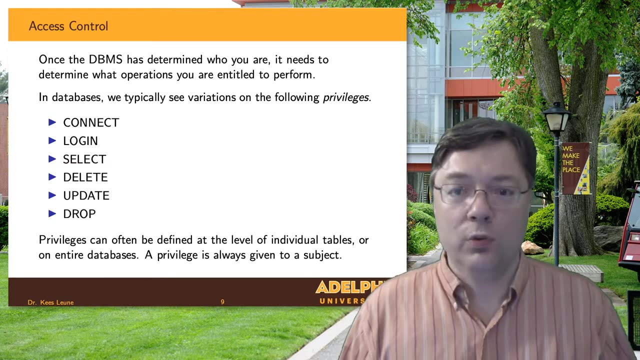 You are maybe not. You are allowed to create new tables in a database, but I might not be. You're allowed to query data in your own database and you might be allowed to query data in one or two of my databases, but that's because I have given you those privileges. 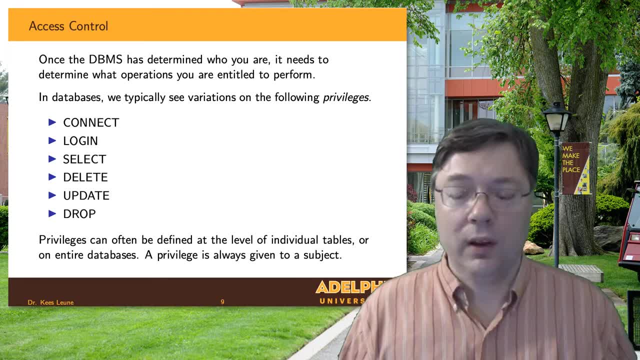 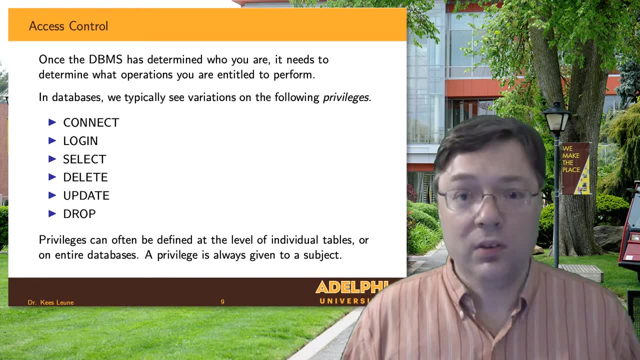 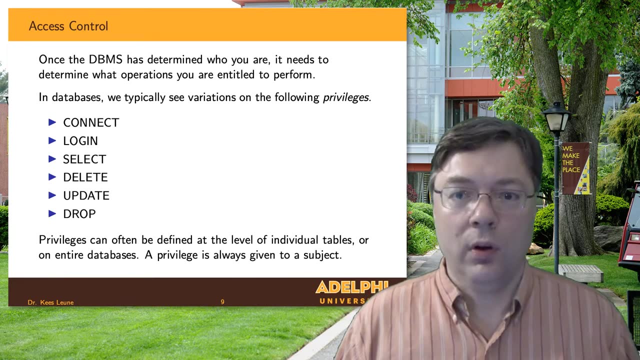 All of those decision points have to be configured, And one of the things we mentioned in the previous video was that many times security falls because misconfiguration. So there's a lot of complexity here. But, for example, when we connect to the database, we need to have some form of an access decision. 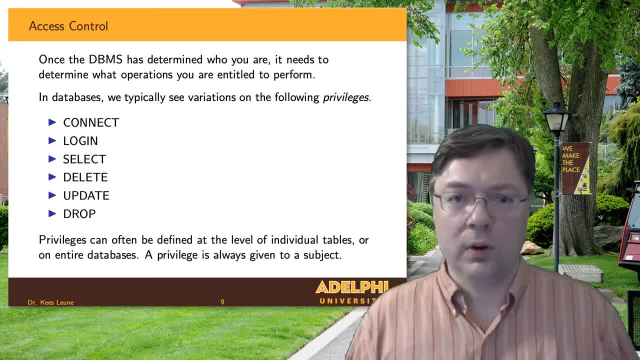 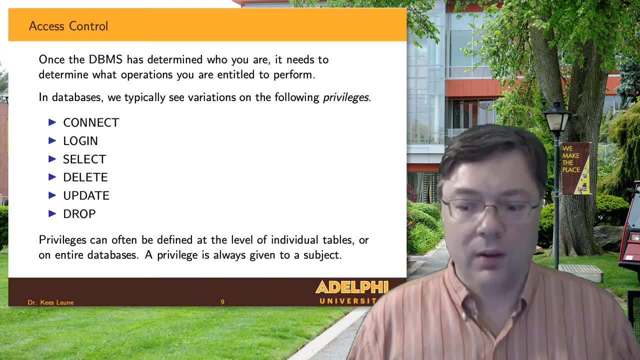 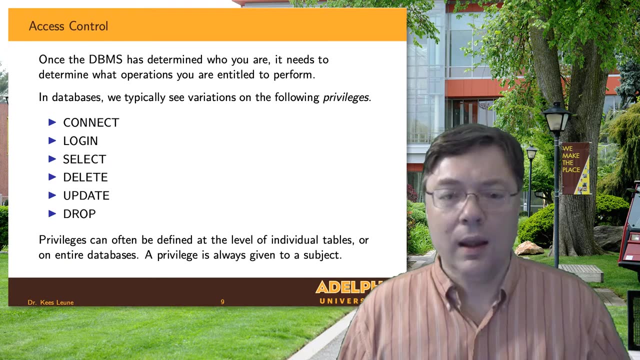 When we then try to log in with usernames and passwords or via some other mechanism, we have to be able to specify policies there. Whether we do select, update, delete, drop operations, create table operations, alter table operations, every single operation can be associated with an explicit permission on the database. 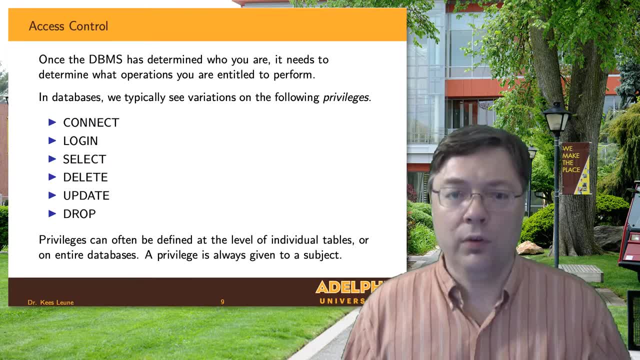 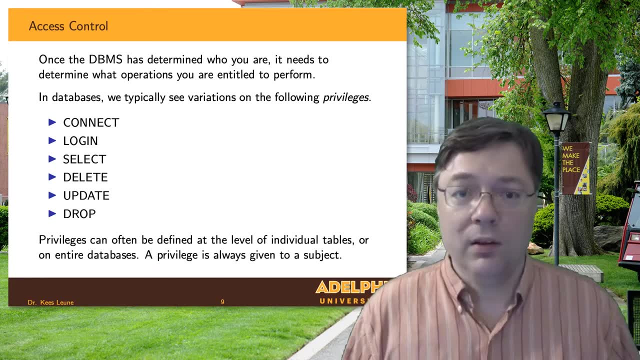 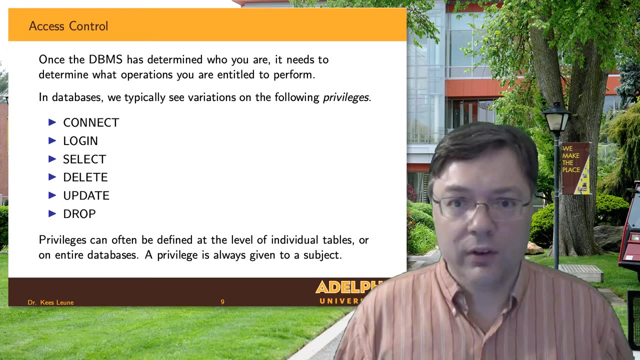 In many cases the permissions are by default configured. really simple: The owner of the database can do everything. Anyone else can do nothing, And that, for sometimes, is sufficient, And in other cases it is not. So these privileges are assigned to subjects or to roles, even better. 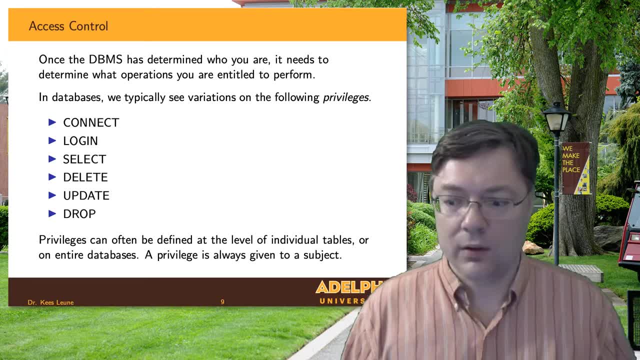 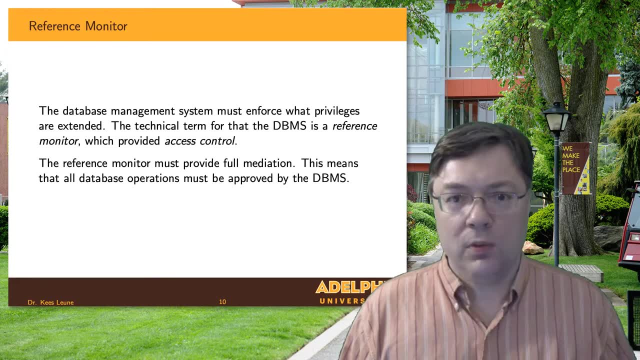 And then the database management system enforces them, And that is called access control. For that to be able to work, all operations through the database management system need to be mediated through something called the reference monitor. The reference monitor must provide full mediation. 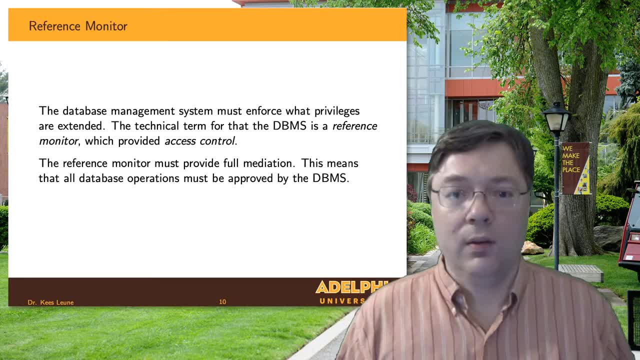 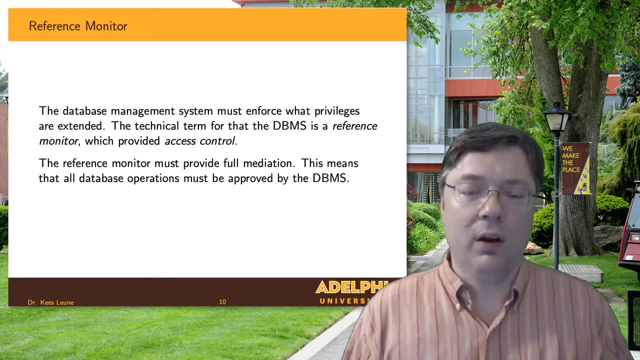 So, in other words, everything you do when you're interacting with the DBMS has to be subject to access control. You shouldn't be able to work your way around that and say, oh you know, I'll just go a different route. 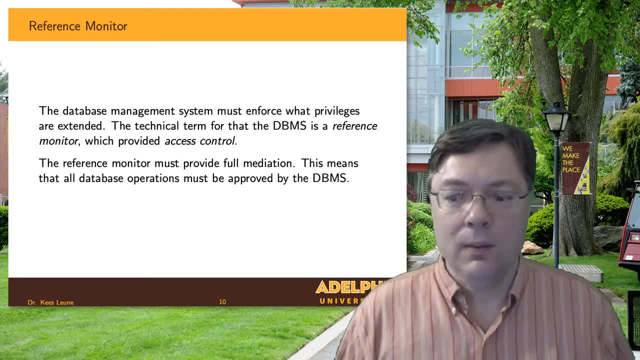 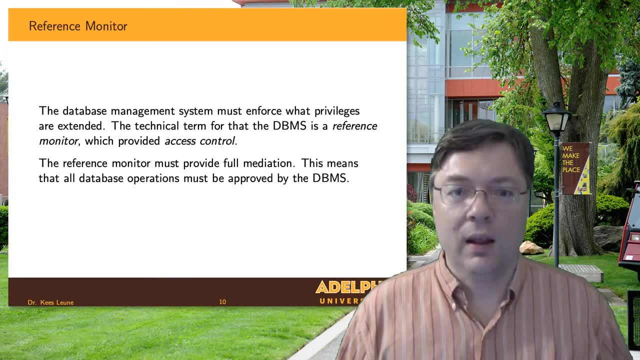 And then I can get in. If that's the case, then you might as well not have these protections in place in the first place. So the reference monitor is the component in the DBMS that enforces authorizations through its access control mechanism. 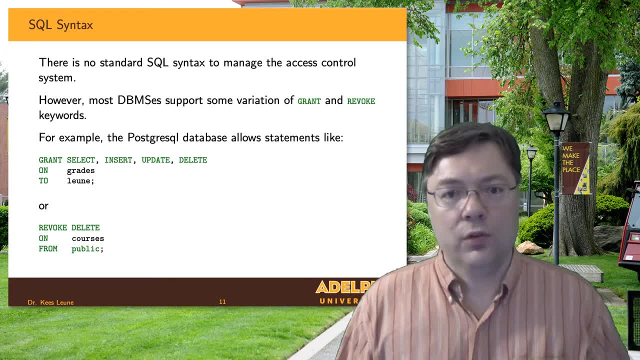 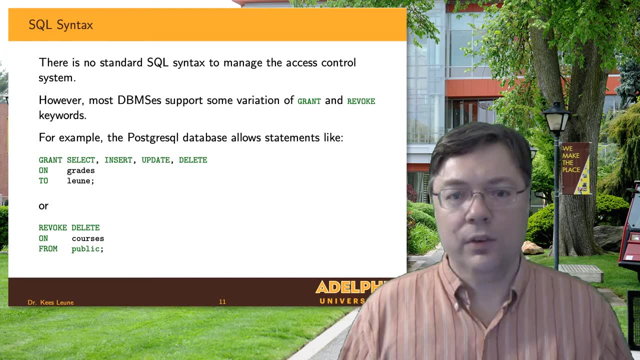 Now, unfortunately in SQL there is no standard syntax to do this. There are very similar variations, but the SQL standard itself does not specify how to do this. Most DBMSs do have a system in place called grant revoke, where the grant statement is used to issue new privileges to new users or new roles. 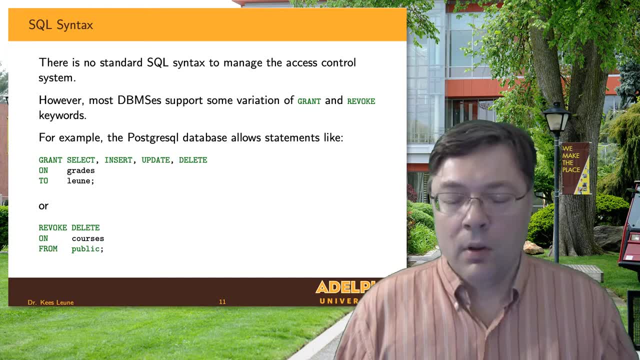 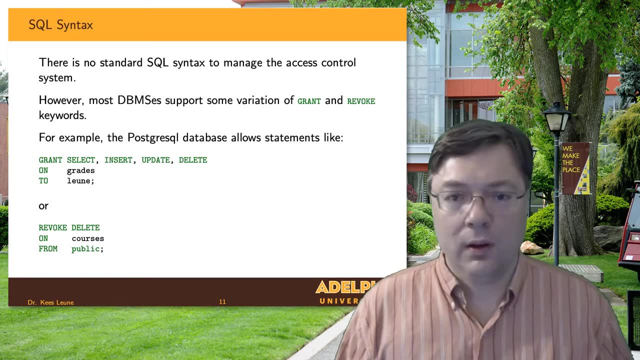 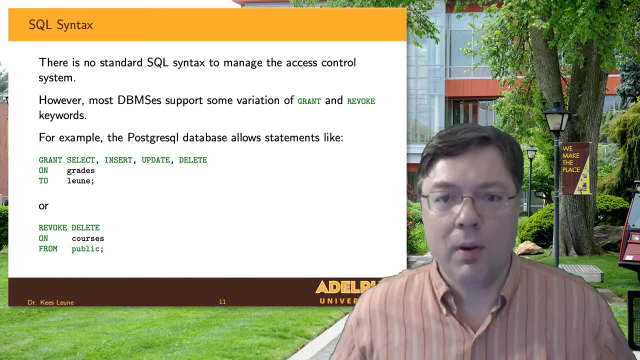 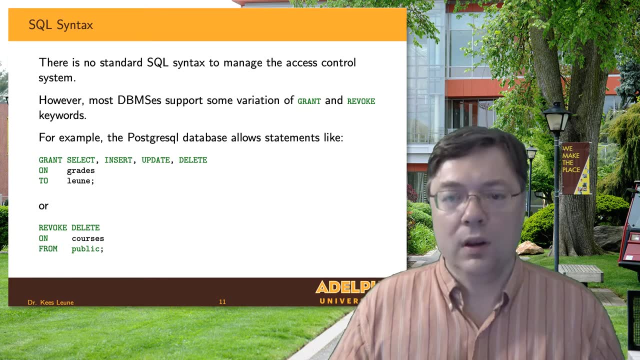 And we'll stick to the PostgreSQL database. But, for example, if I wanted to have my grades table, the one that I create in my database, and I want you to be able to interact with it, I could give you those rights. I could say grant, the key word to give privileges, and then select: insert, update and delete. 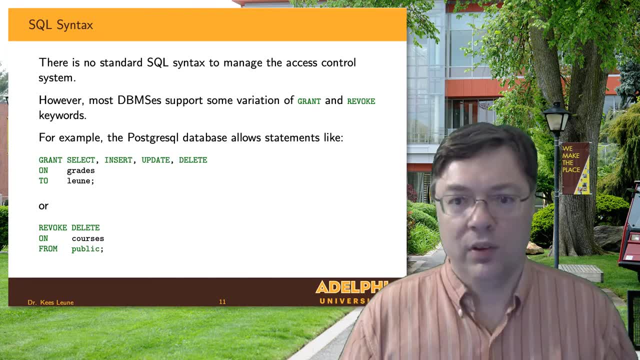 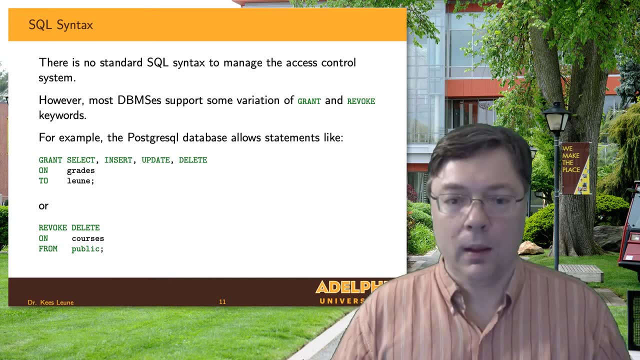 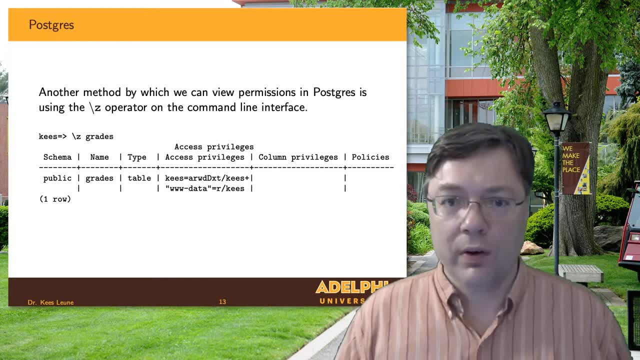 And from that point on that user. in this case I'm giving it to my other account. the learner account will be able to manipulate this table as well If we are in PSQL. so this is a reference monitor command, not a DBMS command. it's backslash Z and then the name of the table. 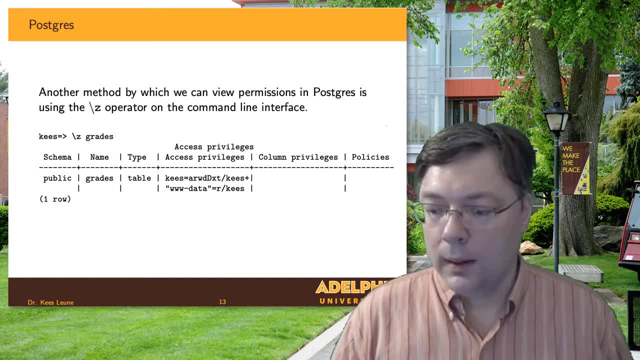 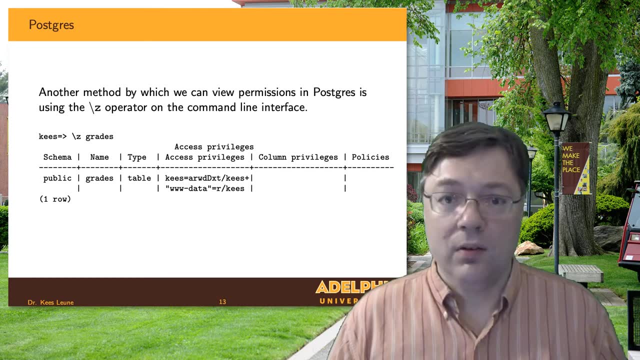 And that gives me the access control list defined on the grades table in this case. So I see that lots of abbreviations are there If you know what they mean. it's a very convenient way. If you don't know what they mean, you'll have to go by syntax and by querying the table. 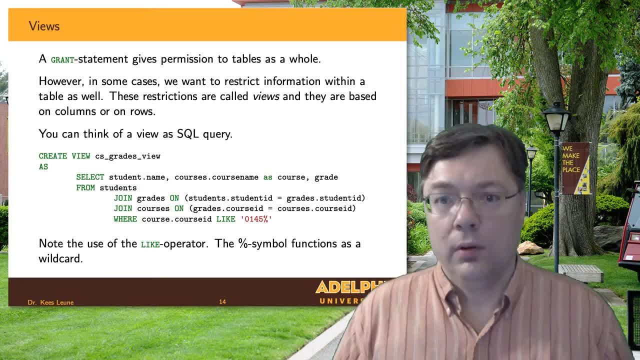 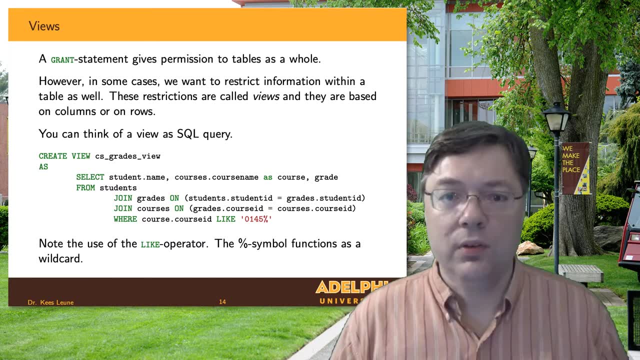 Now, a grant statement or a revoke statement operates on the entire table as one, And that's not always sufficient. There might be situations in which I only want to give access to a particular column in a table, or maybe in particular rows in a table, or a combination of those, And one of the ways I can 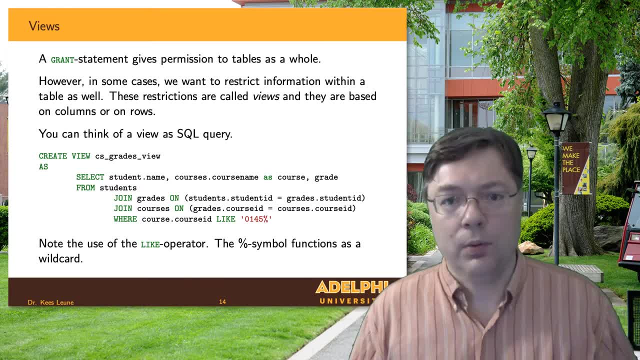 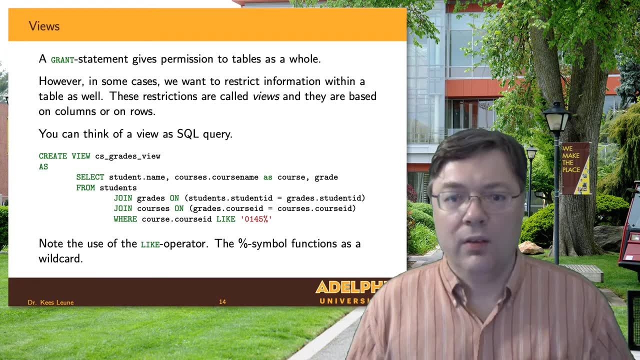 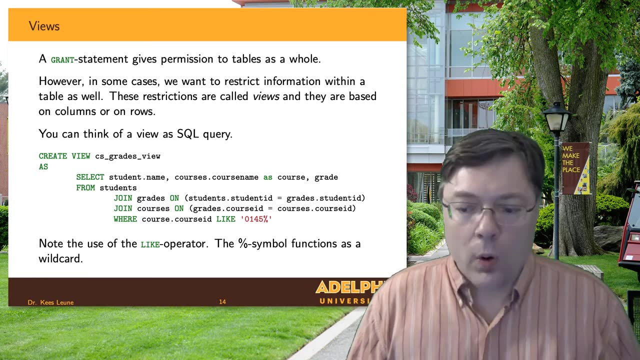 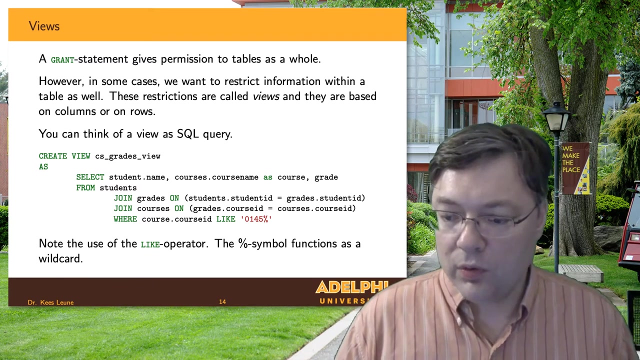 do that is by creating a view and then granting permissions to that view. A view is: think of it as a virtual query. It's a query that creates a temporal table, So I could come up with a query. that's so. the example here: select student name, course name and grade from students. 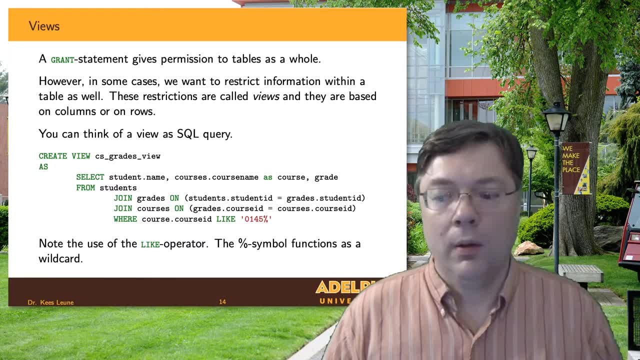 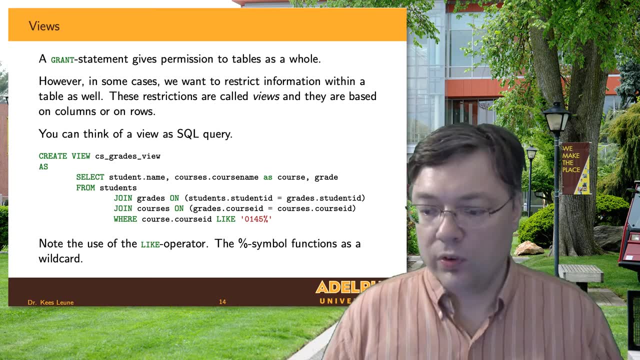 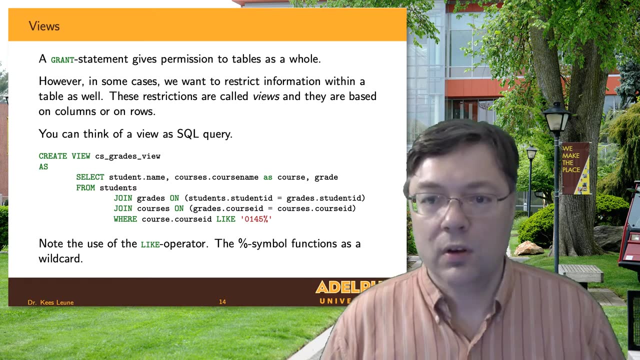 and some join operations and where the course ID like 145.. So, basically, what this query will let me do is query the names, courses and grades from students, as long as they have been graded for a course number that starts with 0145, which, at Adelphi, is the department code. 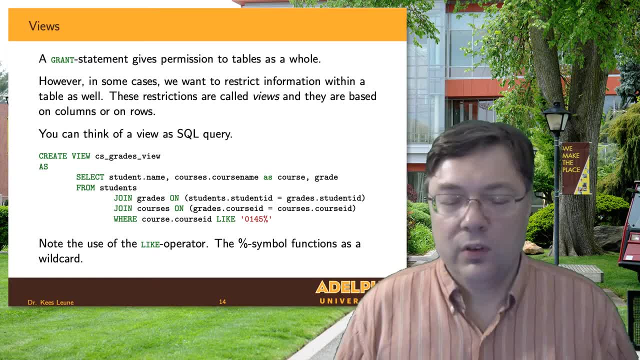 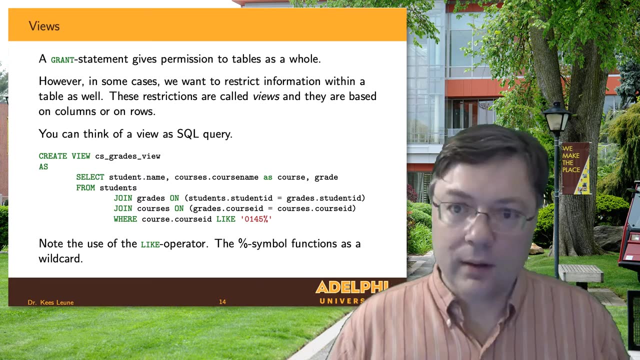 for the computer science program. So in other words, this query will let me figure out who has been graded for computer science courses And I can save that That's called a view, So I can do a create view as a CS, grades view as, and then the query that I run, And now I can query the. 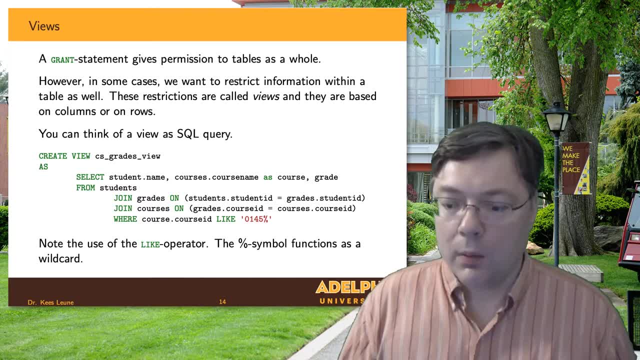 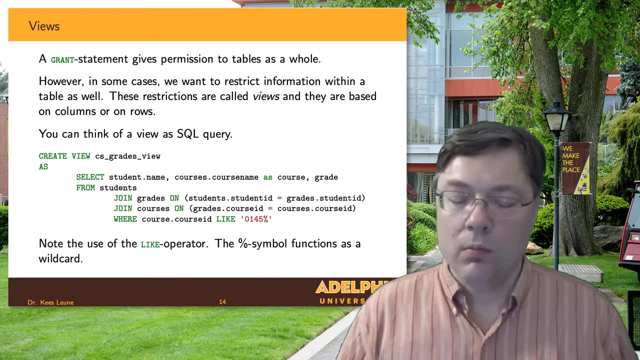 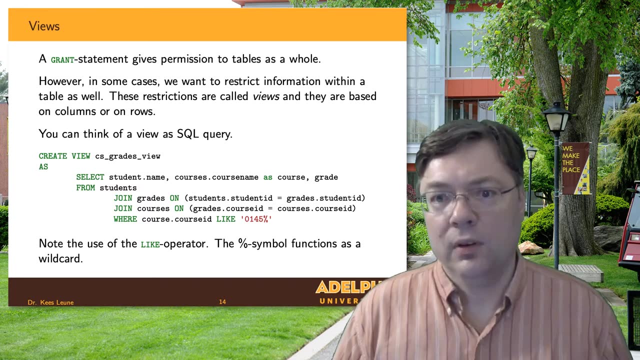 data from this view. So I can do a create view as normal. I can select everything I want from there. Now what I cannot do is update or insert new data from this view. Most view implementations are limited to select only Notice. also, one thing I haven't talked about before explicitly is the 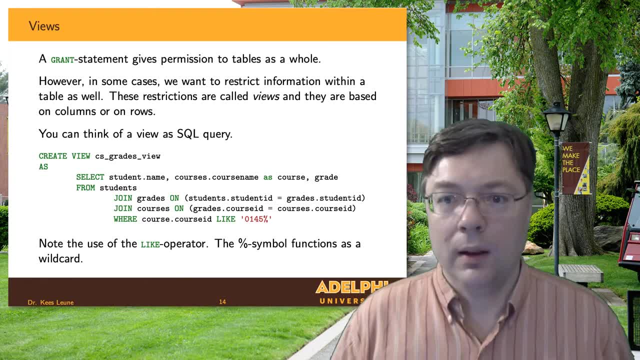 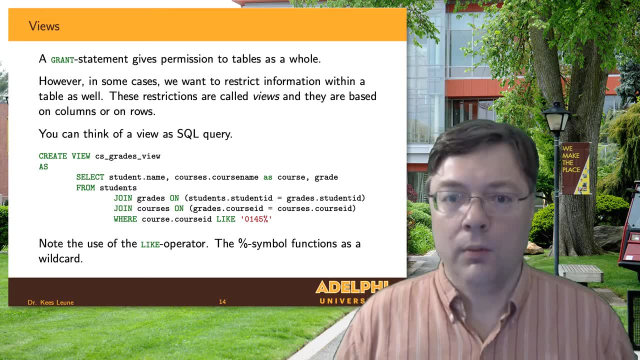 use of wildcards. On the bottom of this query you'll see the word like and then in the text that we're looking for, a percent symbol. If I'm using like, percent becomes a wildcard And that's going to become a placeholder for any possible value. So this is basically stemming 0145 in the 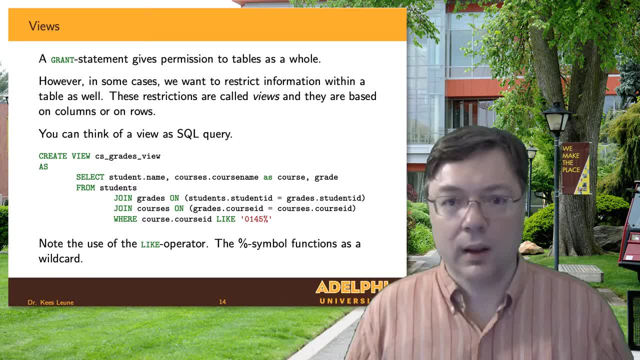 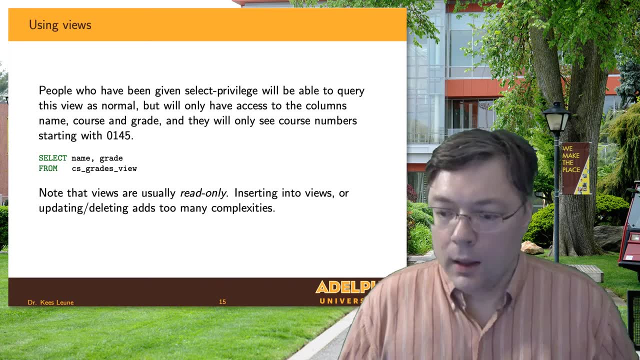 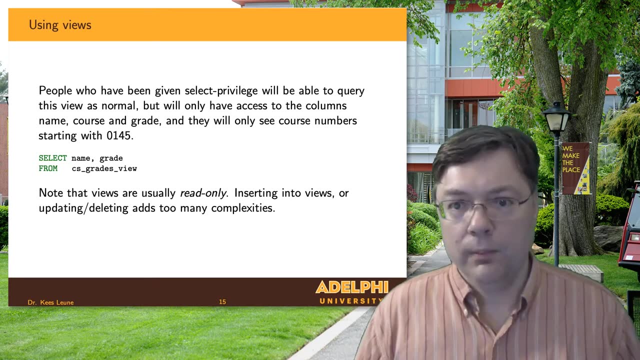 course number And if I use the equals sign, the percent symbol loses its special meaning and it will be a literal match. So if you have the rights on the view, I can query my data. So I could do select name grade from CS grades view very simple, which will then not query CS grades view. it will. 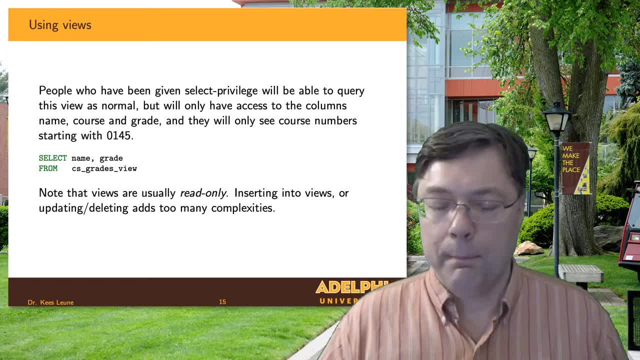 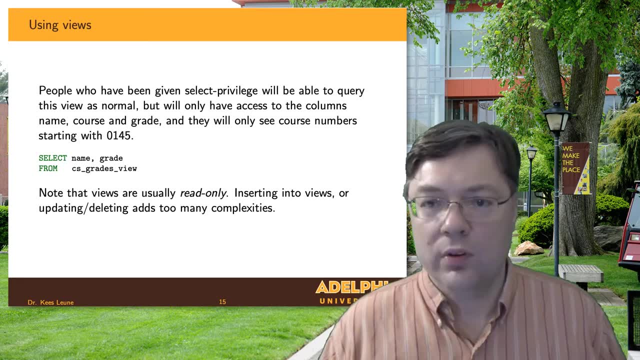 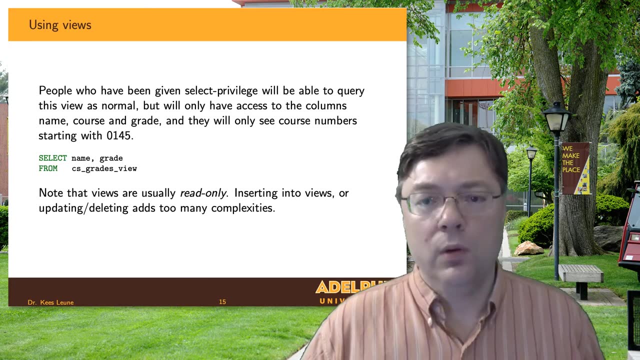 just do the same thing. I can database, do those joints and all of that stuff And that's very convenient. It also, in addition to the use of limiting access to the table or within the table I should say queries can also views can also be used to create backwards compatibility If I change.